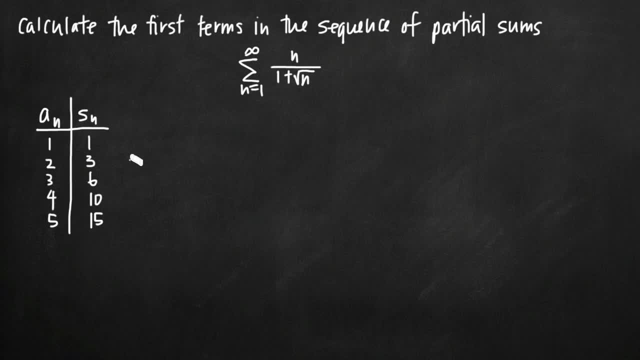 62,, 62,, 68,, 62,, 62,, 65,, 67,, 62,, 63,, 62.. So here we have the regular series, a sub n the series of partial sums We're taking. 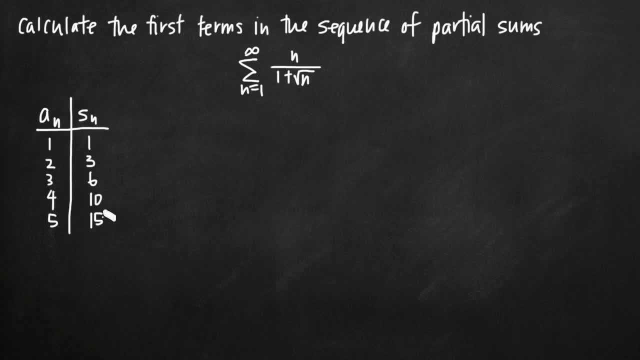 partial sums of this series, In other words, the sum of this series up to the given point. So 10 is the sum of the series up until the fourth term of the series. So that's why we call it the series of partial sums. So in order to calculate the first terms in the 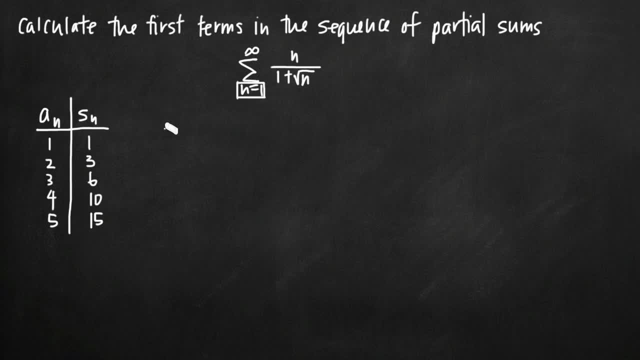 n equals 1.. So we start with n equals 1.. So we say at n equals 1, we plug in 1 to our series here and we get 1 divided by 1 plus the square root of 1.. And of course, when 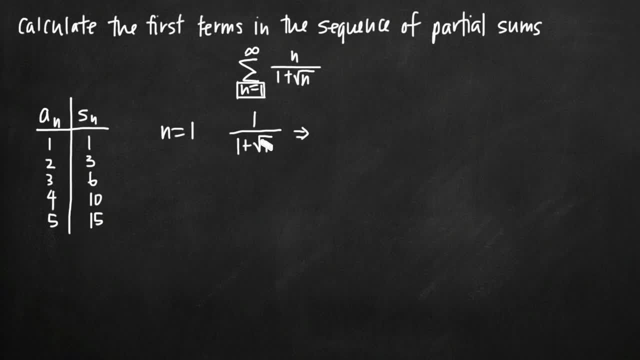 we evaluate that, we'll get the square root of 1 to be 1.. 1 plus 1 is 2., And so we get a value of 1 half, which is equal to 0.5.. And we can just add a couple extra 0's because 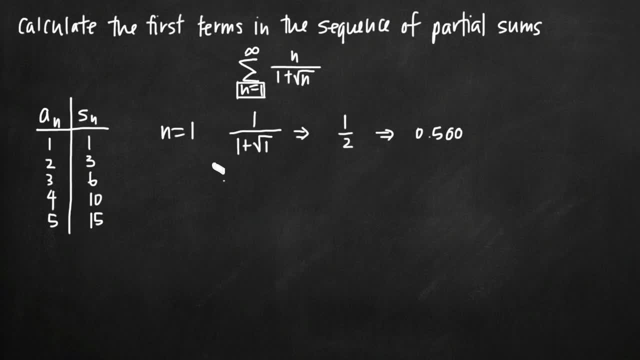 we know we're going to need them later. Okay, so then we plug in a value: n equals 2. And we can just keep doing this right. We'll get 2 divided by 1 plus the square root of 2. And if we evaluate that, we'll get approximately 0.8284.. That's an approximate value, But remember. 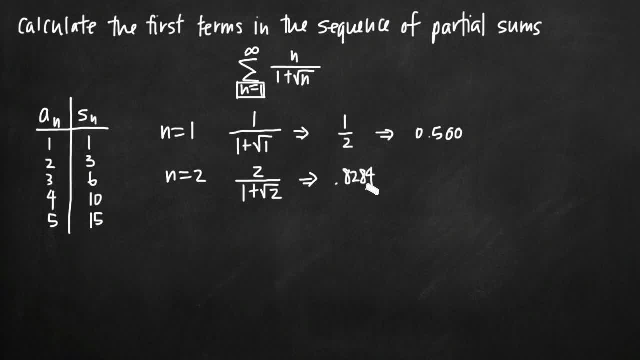 because we're dealing with the sequence of partial sums, we have to add this value, the value of the second term, to the previous term. So we're going to add this value to the previous value that we got. So we have to add that to 0.5.. 0.8284 plus 0.5 is going. 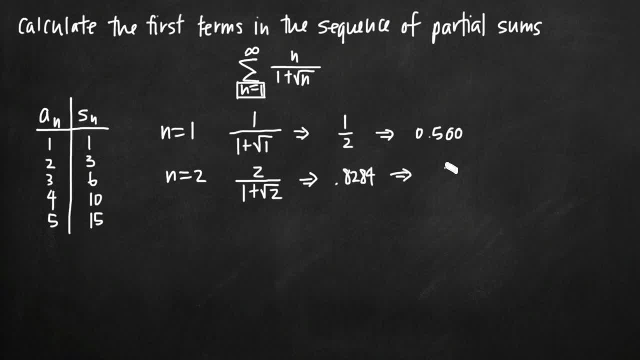 to give us the value of the second term in the sequence of partial sums, which is approximately 1.3284.. And we can round that to about 328.. So let's just do one more term. We'll get n equals 3.. We'll get 3 over 1 plus the square root of 3.. When we evaluate that on, 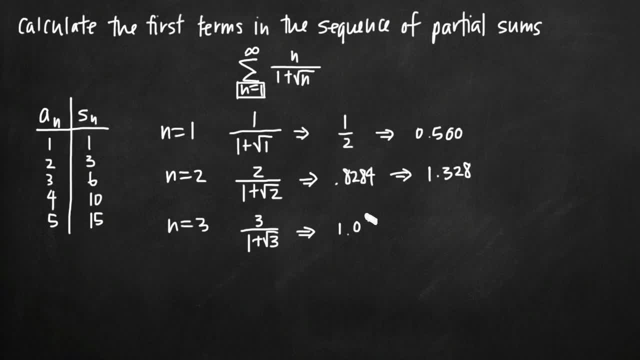 our calculator we'll get approximately 1.098 or so. But remember that's only the third term of a sub n. In order to get the third term of s sub n, we need to add it to our previous value of 1.328.. When we do that and we round, we get approximately 2.427 for the